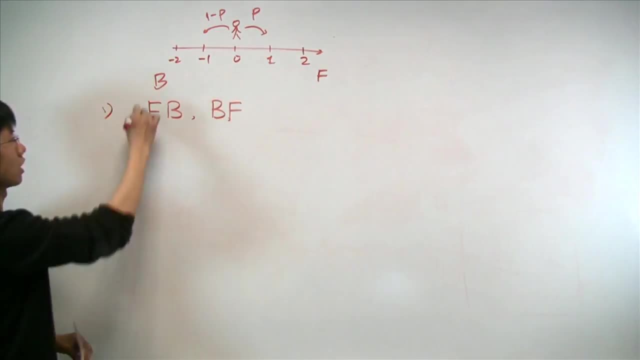 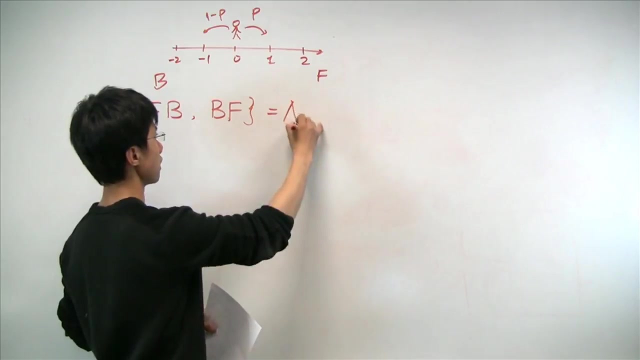 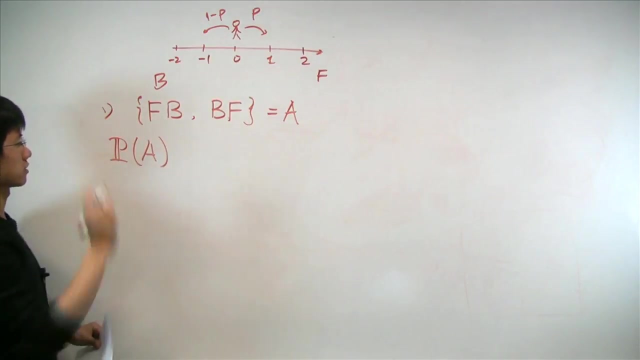 or backward, followed by forward, And indeed this event, namely the union of these two possibilities, defines the event of interest in our case, And we'd like to know what's the probability of A which will break down into the probability of forward. 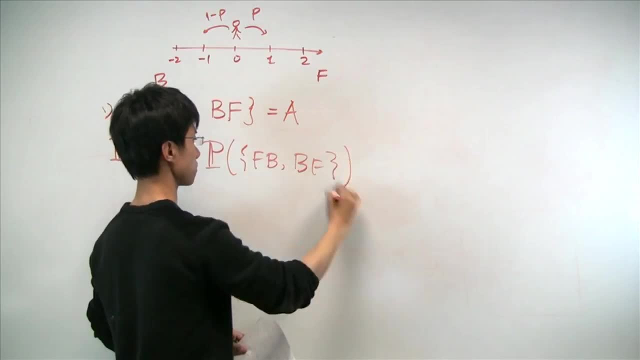 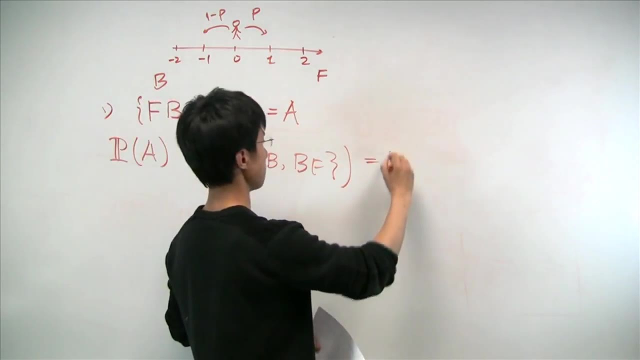 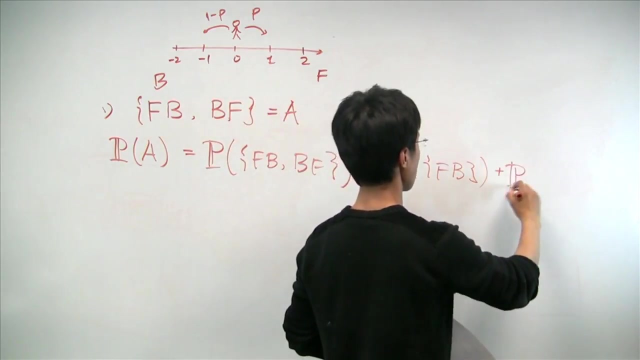 backward, backward forward. Now, forward, backward and backward forward. they're two completely different outcomes And we know that because they're disjoint. this will just be the sum of the two probabilities plus probability of backward forward. 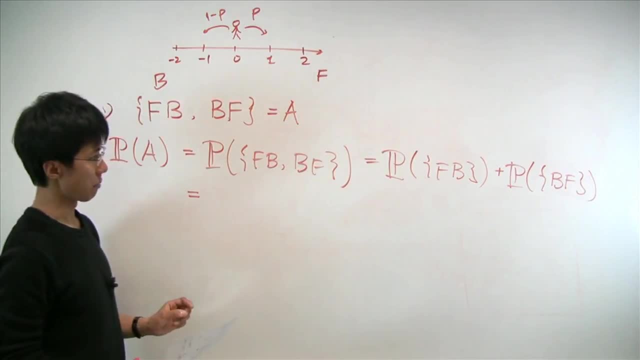 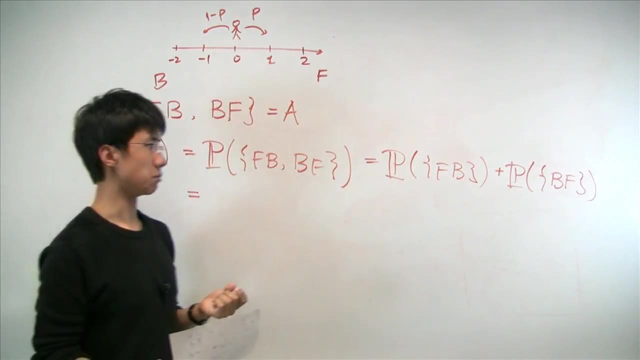 Here's where the independence will come in. When we try to compute the probability of going forward and backward- because the action in this case, in each step, is completely independent from the past- we know this is the same as saying in the first step. 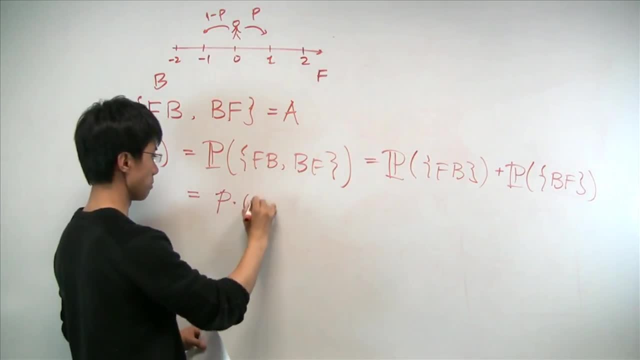 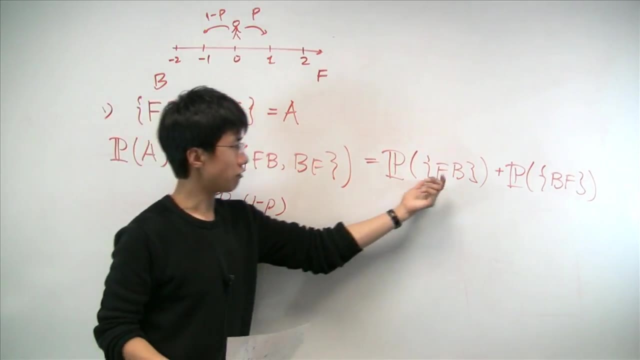 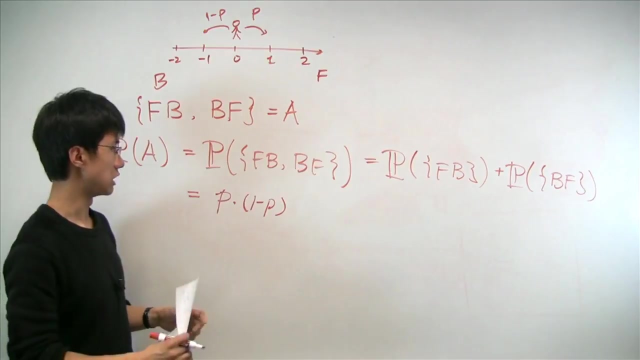 we have probability p of going forward in the next step, probability 1 minus p of going backwards. We can do so, namely writing the probability of forward backward as a product of going forward times the probability of going backwards, because these two actions are independent. 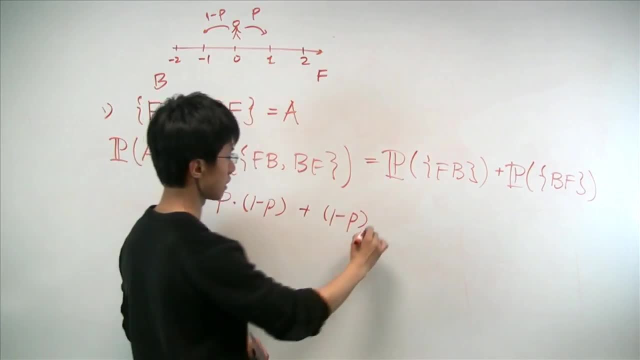 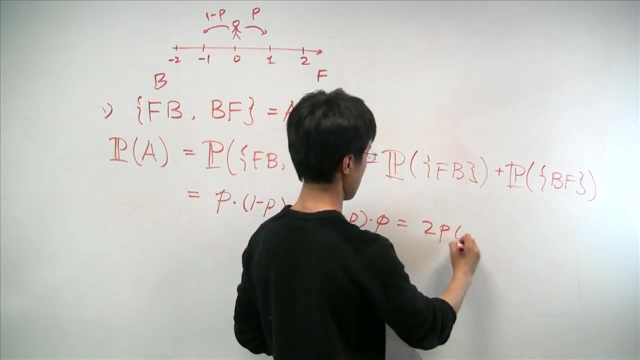 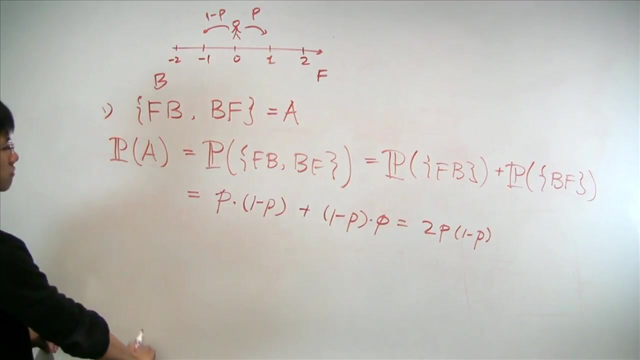 And similarly for the second one. we have going backwards first times, going forward forward the second time. Adding these two up, we have 2 times p, times 1 minus p, And that will be the answer to the first part of the problem. In the second part of the problem we're interested in, 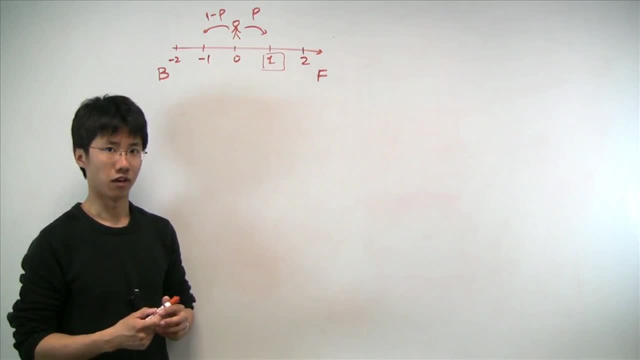 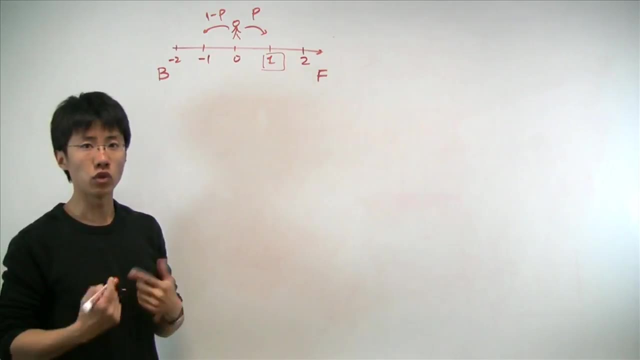 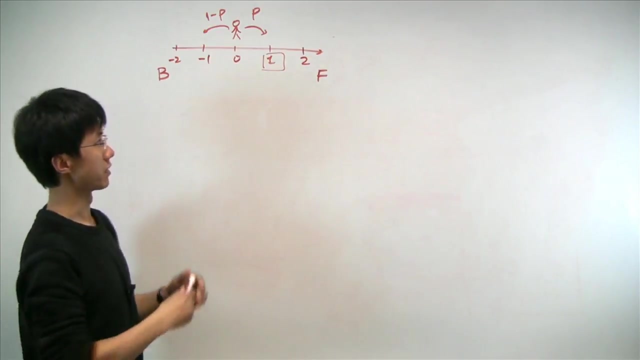 the probability that after three steps, the person ends up in position 1 or one step forward compared to where he started. Now the only possibilities here are that among the three steps, exactly two steps are forward and one step is backward, because otherwise there's no way the person will. 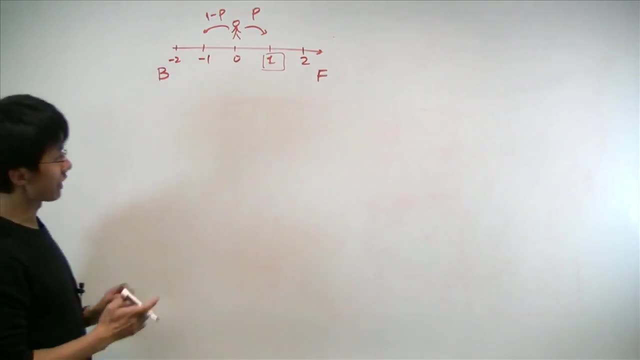 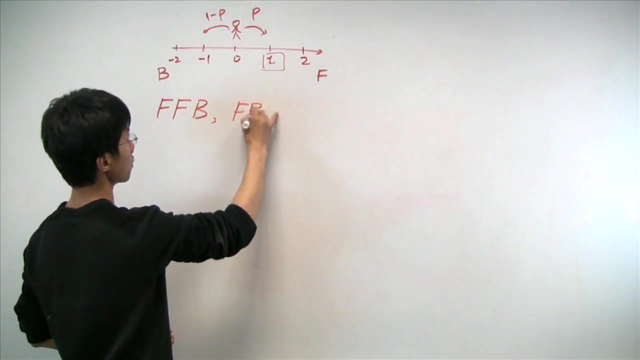 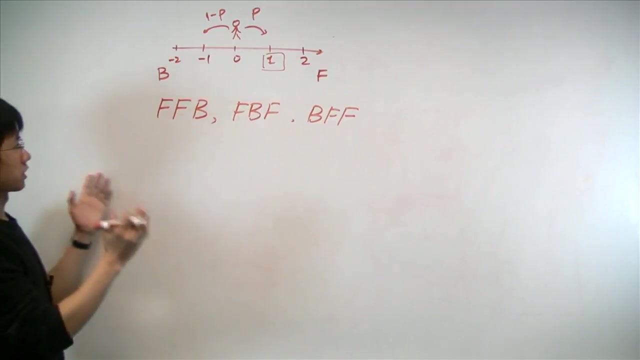 end up in position 1.. To do so, there again are three possibilities in which we go forward, forward, backward, or forward, backward, forward or backward forward, forward. And that exhausts all the possibility that the person can end up in position 1 after three steps, And we'll define the. 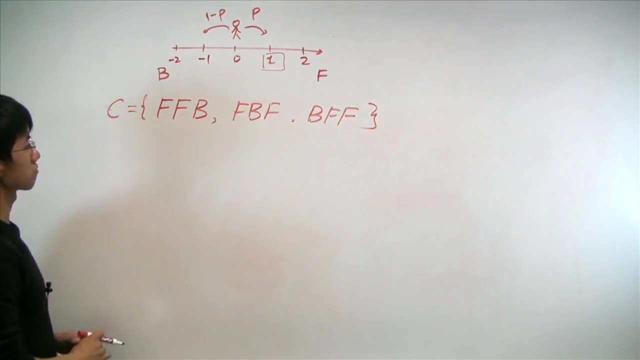 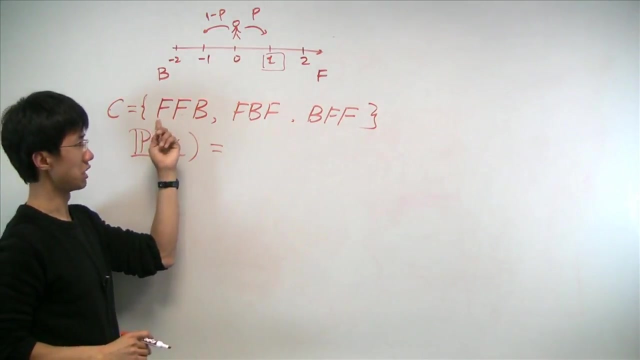 collection of all these outcomes and the probability that the person will end up in position 1 after three steps. The probability of this is the same as the probability of event C. The probability of event C, same as before, is simply the sum of the probability of each individual outcome. Now, 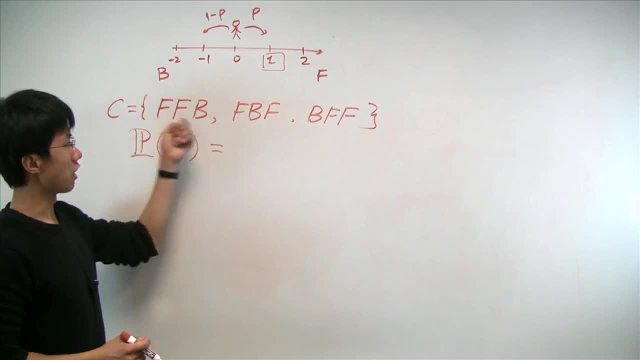 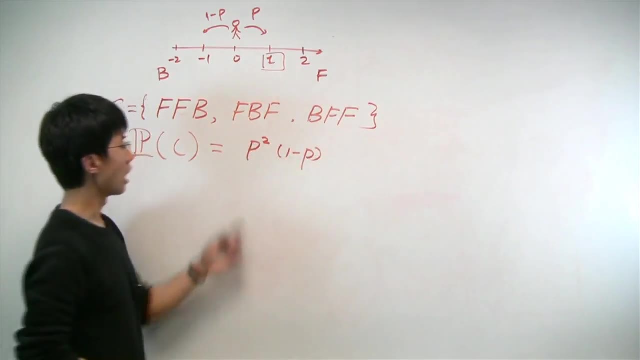 based on the independence assumption that we used before, each outcome here has the same probability, which is equal to p squared times one minus p. The p squared comes from the fact that two forward steps are taken, and y minus p the probability of that one forward step In the future. one of these comes from the handling of the example that I just basically picked up, and all of these become pre-published outcomes. So this is a real problem of this. This is the code that goes on in this particular document, So we've got two steps forward and then a step forward, and 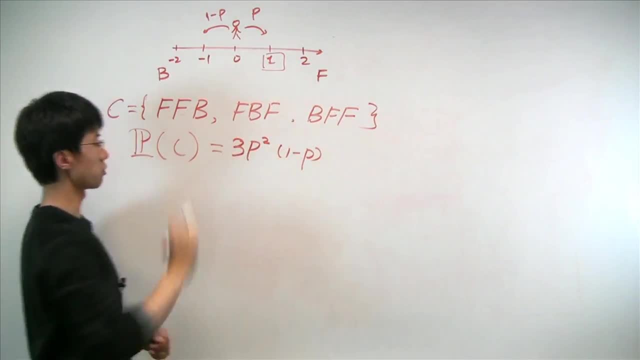 two steps backward come in. So we need one step forward and two steps backward And one step back and one step forward step and since there are three of them, we multiply three in front and that will give us the probability. 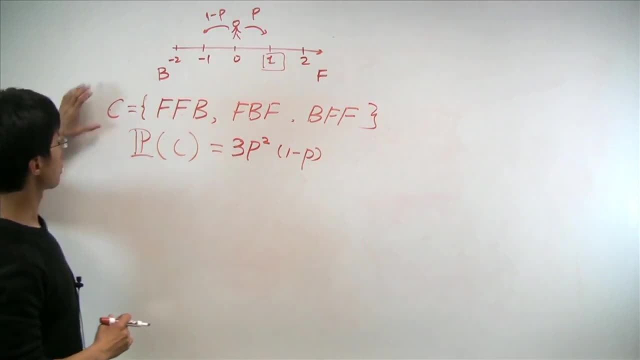 In the last part of the problem we're asked to compute that conditional on event C already took place. What is the probability that the first step he took was a forward step? Without going into the details, let's take a look at the C, in which we have three elements. 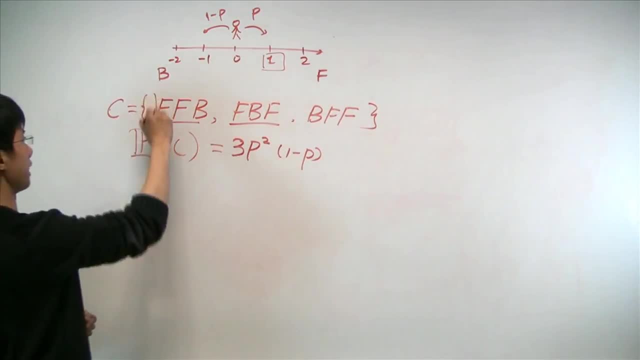 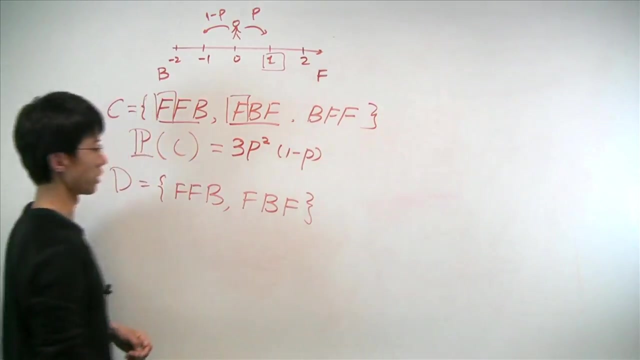 and only the first two elements correspond to a forward step in the first step. So we can define event D as simply the first two outcomes: forward, forward backward and forward backward forward. Now the probability we're interested in is simply probability of D conditional on C. 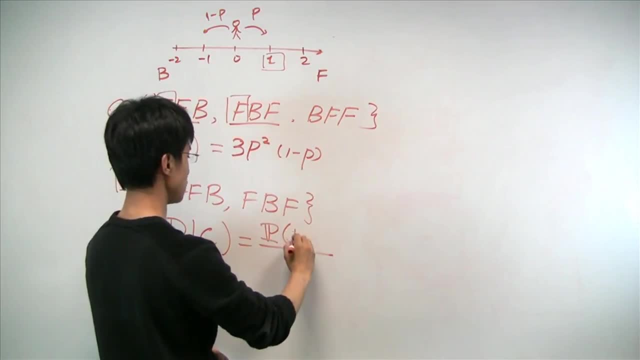 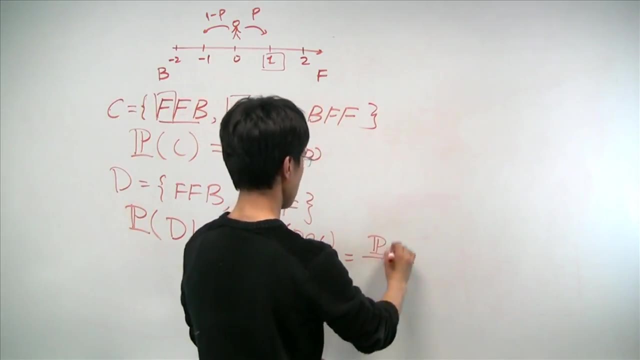 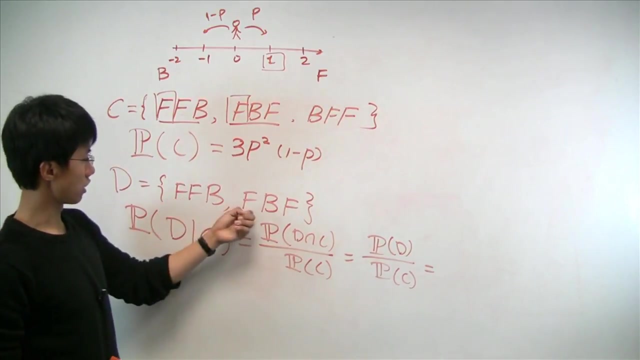 We write it out using the law of conditional probability: D intersection C, conditional on C. Now, because D is a subset of C, we have probability D divided by the probability of C. Again, because all samples here have the same probability, all we need to do is to count the number of samples here, which is two, and divide by. 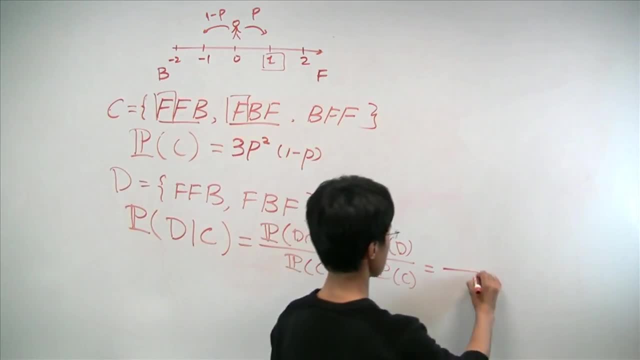 the number of samples here, which is three. So we end up with three, two over three, And that concludes the problem. See you next time.